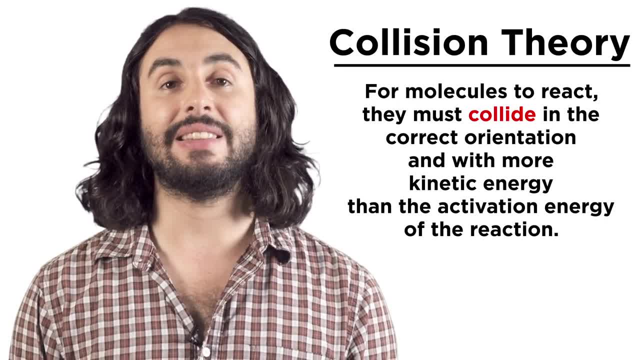 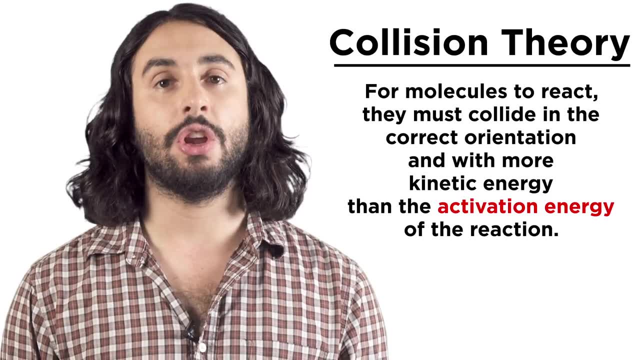 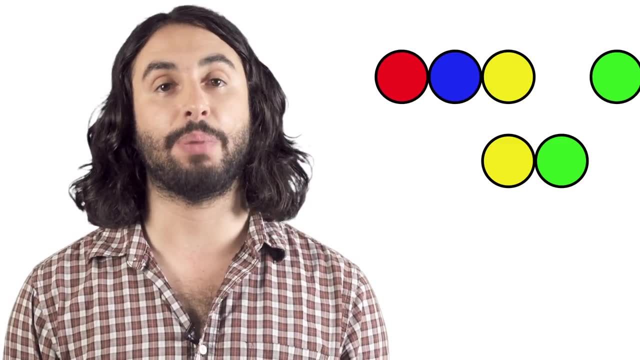 and with an amount of kinetic energy that exceeds the activation energy of a reaction. this is the amount of energy that has to be provided to allow for the reaction to proceed. here we can see that the two molecules have to collide in a particular way in order to react, otherwise they will bounce right off each. 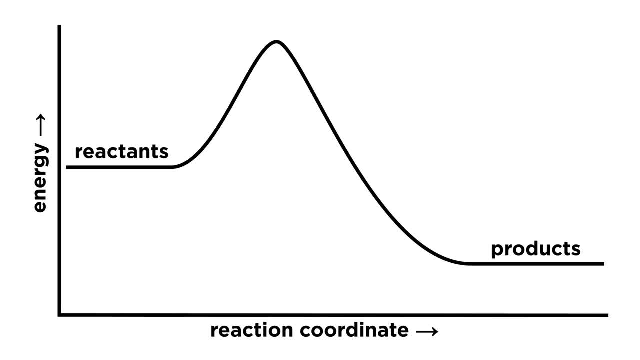 other. as for energy, let's refer to an energy diagram on. these up means higher energy and to the right means later in time. so we can see that any reaction will have an activation energy, which is the kinetic energy that the molecules must collide with in order to reach the transition state. this is the orientation which once 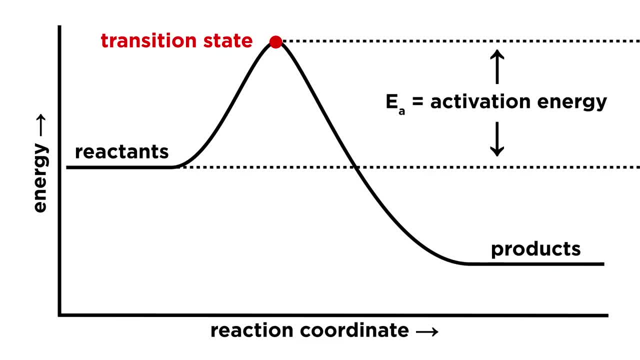 reached, the reaction will certainly occur. collisions with less energy than this will not result in a reaction. from energy diagrams we can also see delta H, or the difference in energy between the reactants and products. if the products sit lower, it is an exothermic reaction which releases energy. if the products 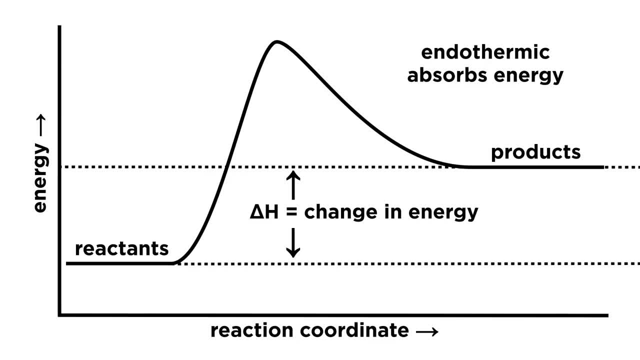 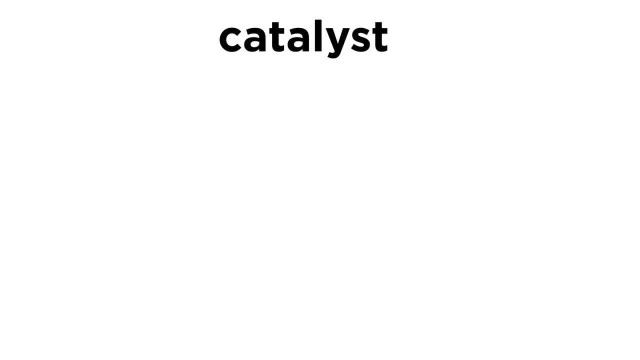 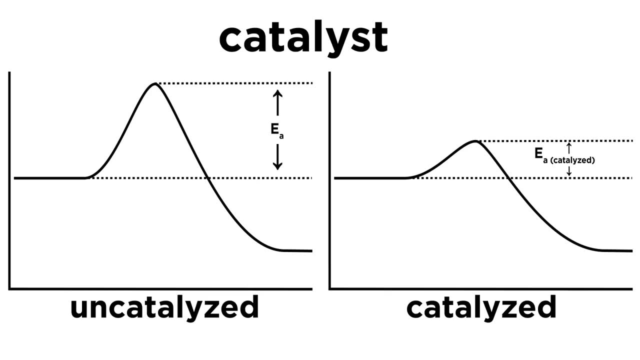 sit higher. it is an endothermic reaction and needs to absorb energy to occur. most people would refer to a catalyst as something that speeds up a reaction. while this is often true, the better definition is that a catalyst is something that lowers the activation energy. 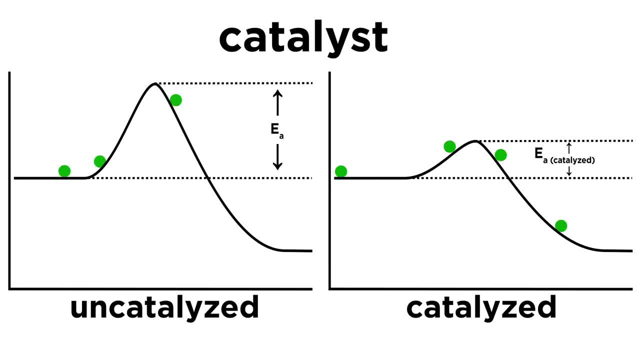 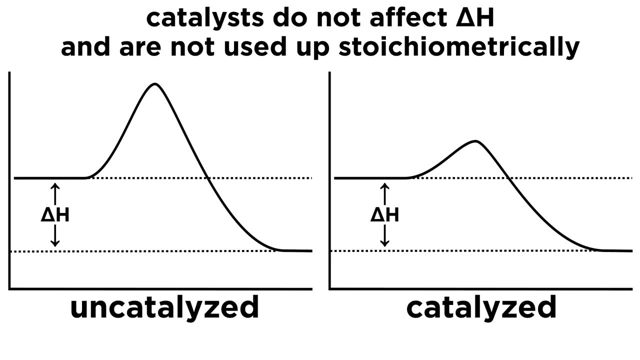 of a reaction because the activation energy is lower, many more collisions will result in a successful reaction, which is why catalysis typically results in a faster rate of reaction. catalysts do not affect the delta H of a reaction and they are not used up stoichiometrically in a reaction in other. 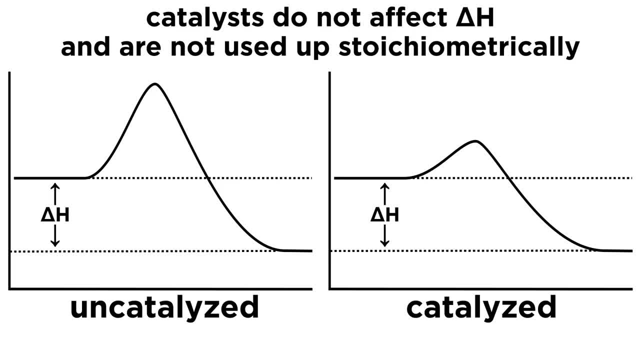 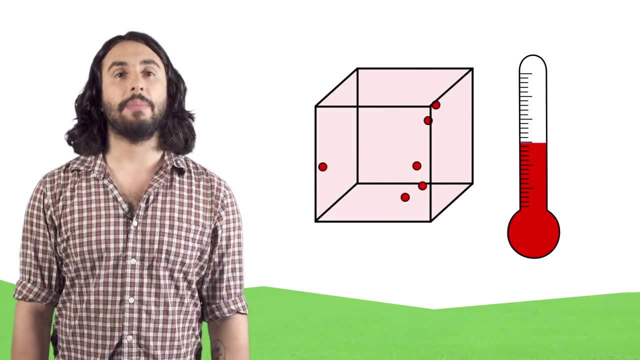 words, one molecule of catalyst can facilitate many, many reactions, unlike molecules of reactant, which are used up in order to make products. reactions also tend to have faster rates at higher temperatures, because more heat energy means faster moving molecules, which means more kinetic energy at higher 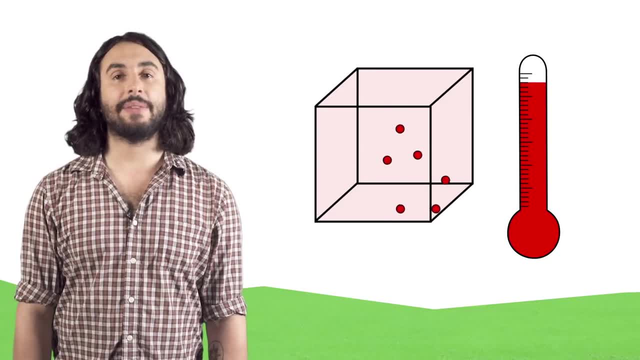 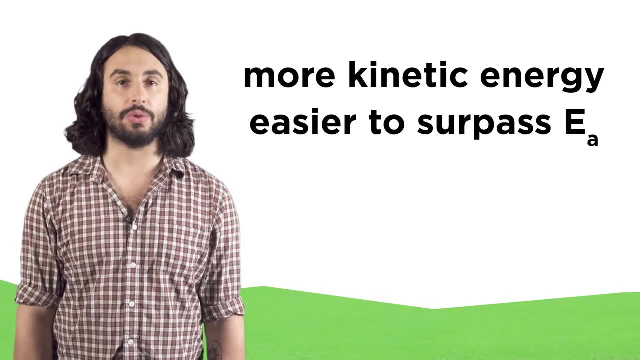 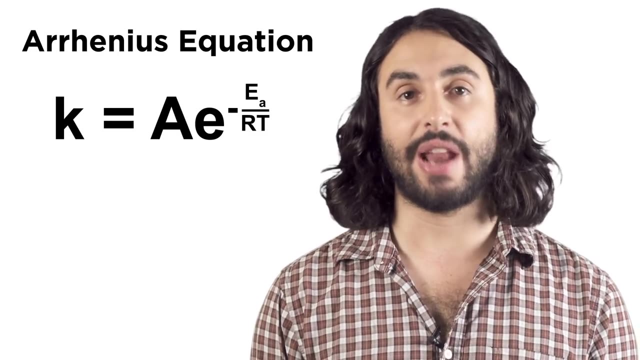 temperatures. more individual collisions will have sufficient energy to surpass the activation barrier, so the overall reaction for many trillions of molecules will proceed more quickly. the Arrhenius equation shows how the rate constant depends on the activation energy. in this equation, A is a constant called the. 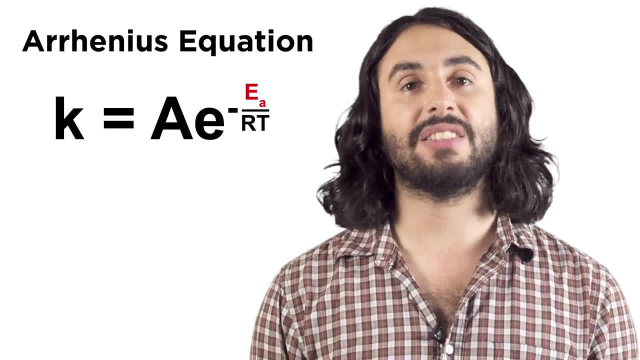 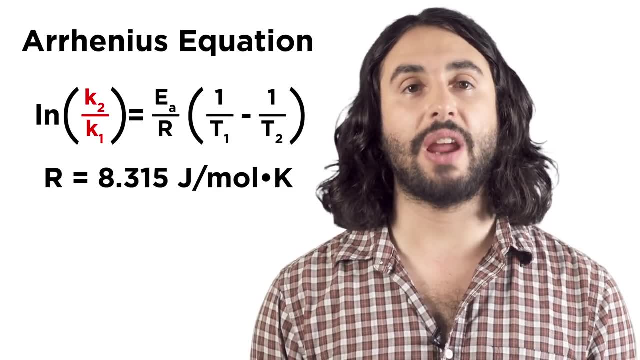 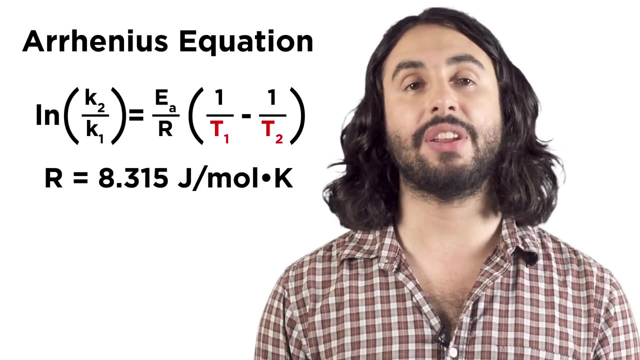 frequency factor and we have the number E, the activation energy and the gas constant, as well as temperature. this equation can be modified to show the ratio of the rate constant for a reaction at two different temperatures. this is the one that we can use to calculate the activation energy of 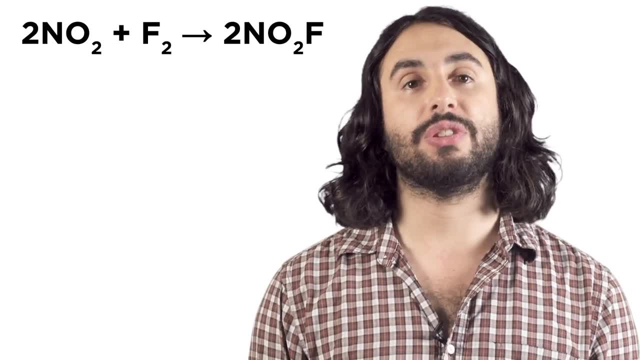 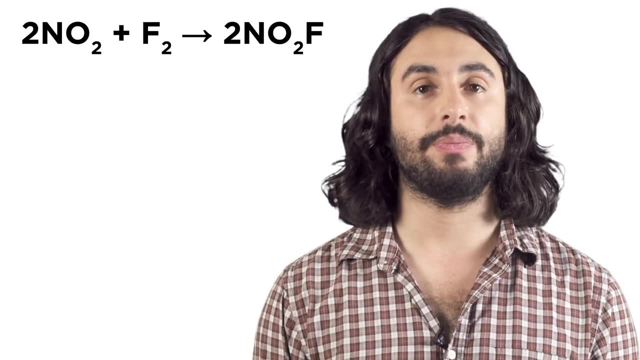 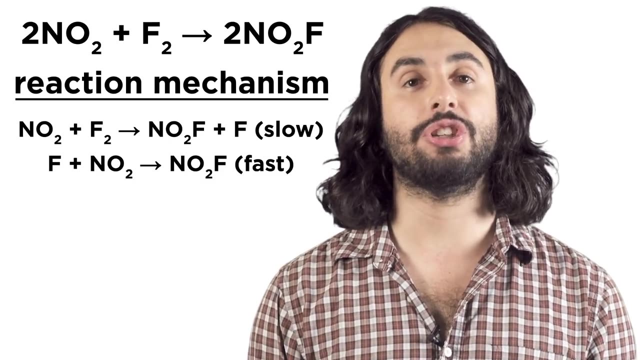 a reaction. a balanced chemical equation will tell you the starting materials and products of a reaction, but sometimes what is happening on the molecular level is more complicated than this. the series of steps that actually occurs is called the reaction mechanism for the following reaction. we can break it down into: 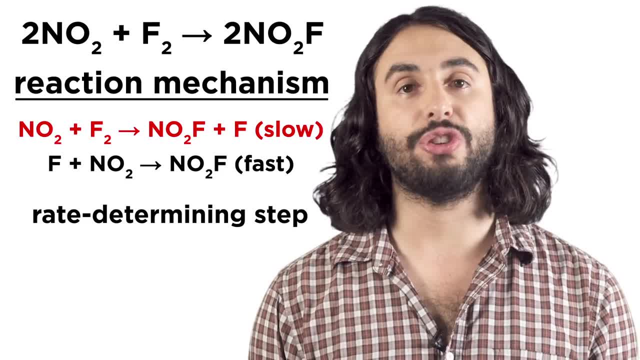 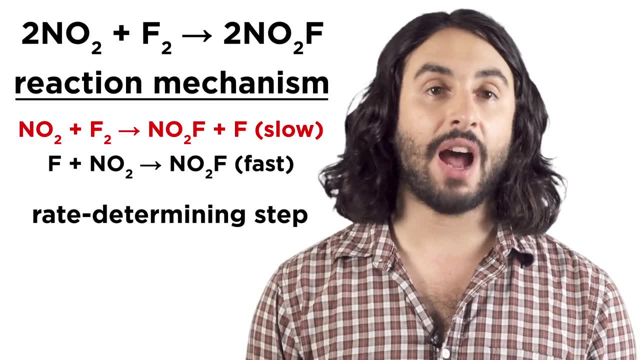 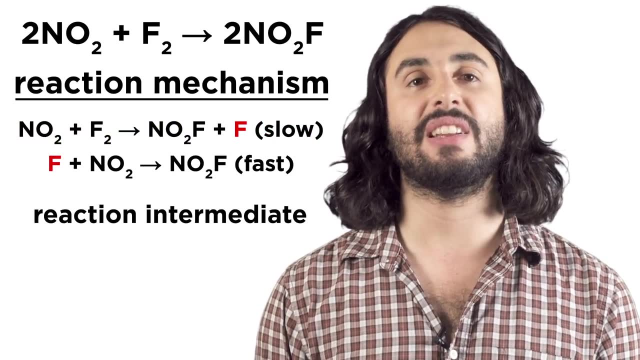 elementary steps. the slowest step is called the rate determining step, because the rate predominantly depends only on this step, as the other step or steps are so much faster that they are negligible in comparison. a species that is found in elementary steps but not in the overall equation is called a reaction. 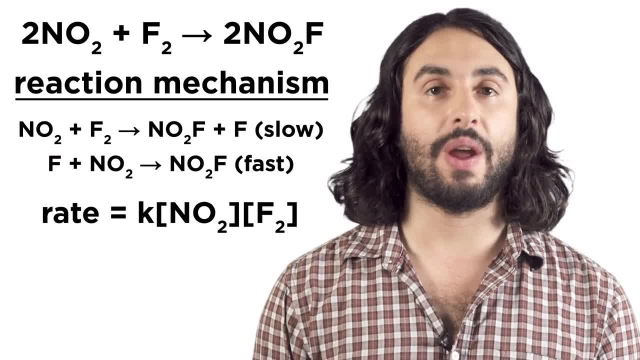 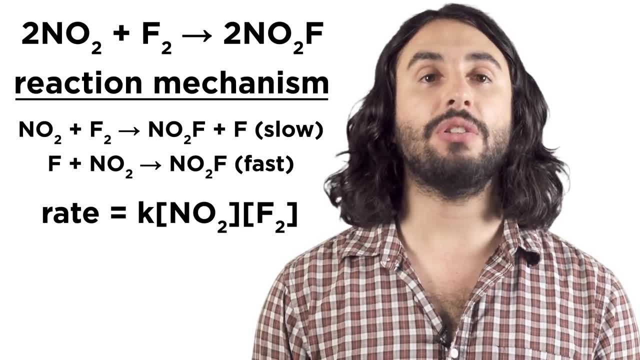 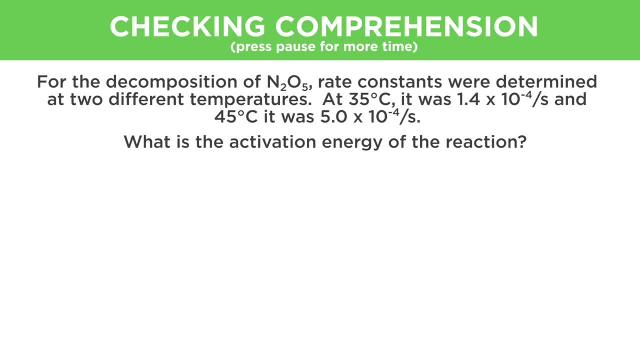 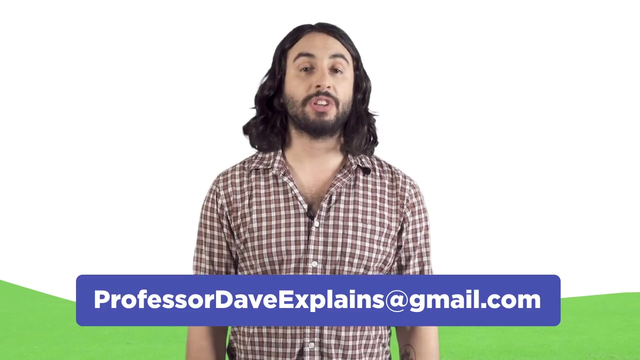 intermediate. the rate law for the overall equation can be discerned directly from the rate determining step and by this method the exponents will equal the stoichiometric coefficients. let's check comprehension. thanks for watching, guys. subscribe to my channel for more tutorials and, as always, feel free to email me. professordaveexplains at gmailcom.